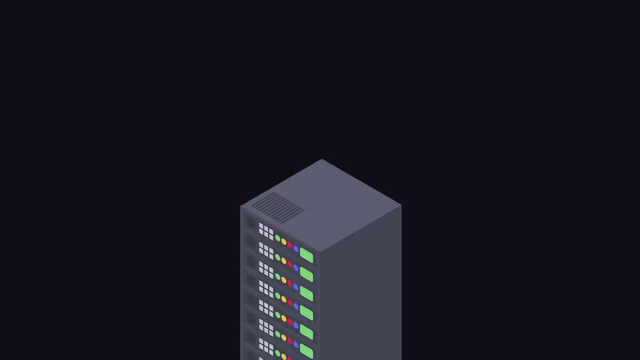 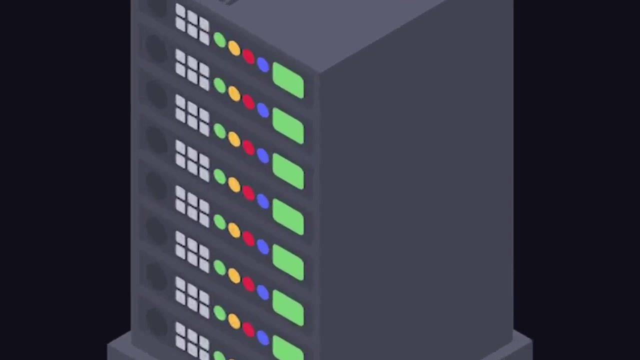 The big question is: how do we scale our infrastructure? A server can scale up into vertically or horizontally. To scale vertically, you take your one server and increase its RAM and CPU. This can take you pretty far, but eventually you hit a ceiling. The other option is to scale. 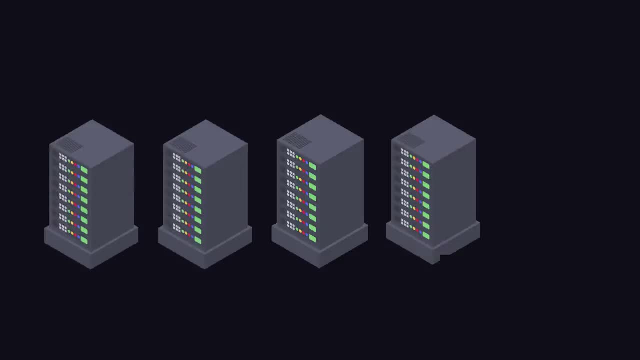 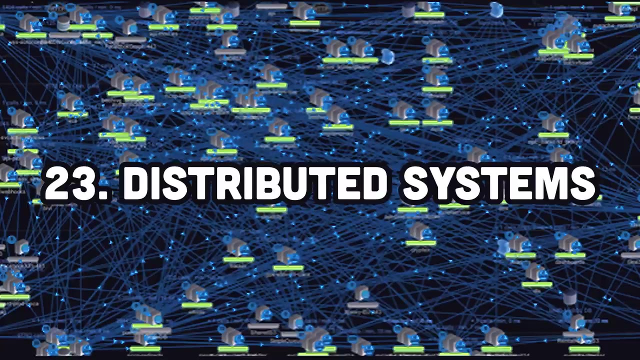 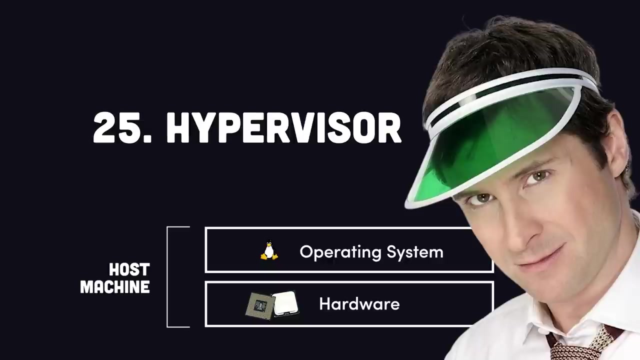 horizontally, where you distribute your code to multiple smaller servers, which are often broken down into microservices that can run and scale independently. But distributed systems like this aren't very practical when talking about bare metal, because actual resource allocation varies. One way engineers address this is with virtual machines. using tools like Hypervisor It can. 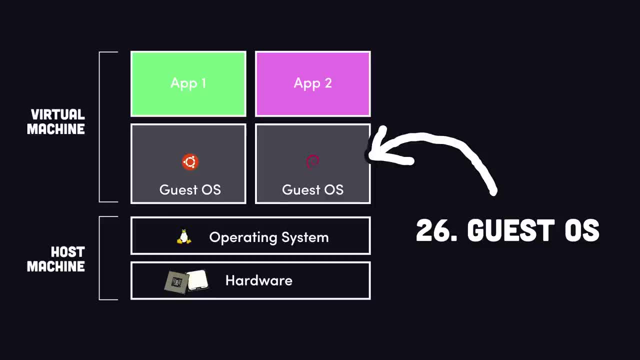 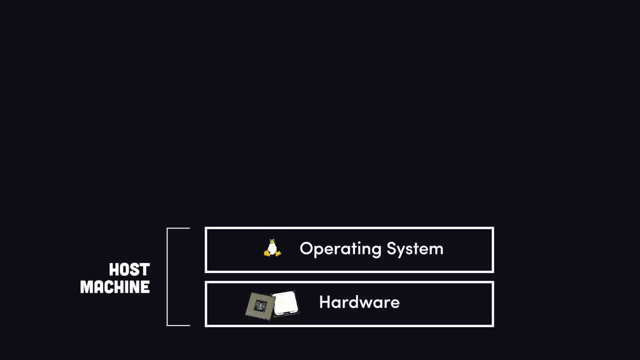 simulate and run multiple operating systems on a single machine. That helps, but a VM's allocation of CPU and memory is still fixed, And that's where Docker comes in. The sponsor of today's video. Applications running on top of the Docker engine all share the same host operating. 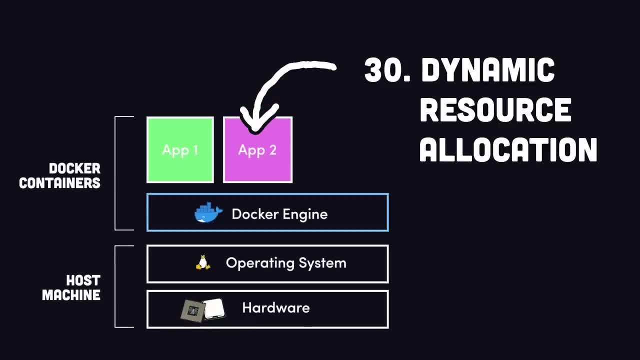 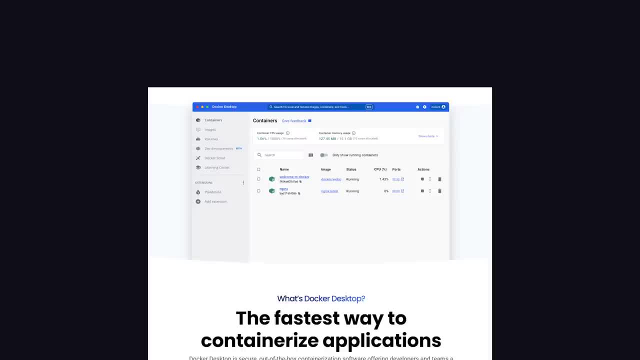 system kernel and use resources dynamically based on their needs. Under the hood, Docker's running a daemon or persistent process, that makes all this magic possible and gives us OS-level virtualization. What's awesome is that any developer can easily harness this power by 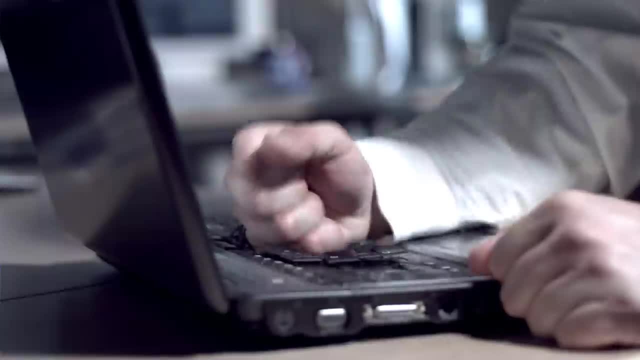 simply installing Docker Desktop. It allows you to run multiple operating systems on a single machine and it allows you to develop software without having to make massive changes to your local system. But here's how Docker works, in three easy steps. First, you start with a Docker file- This: 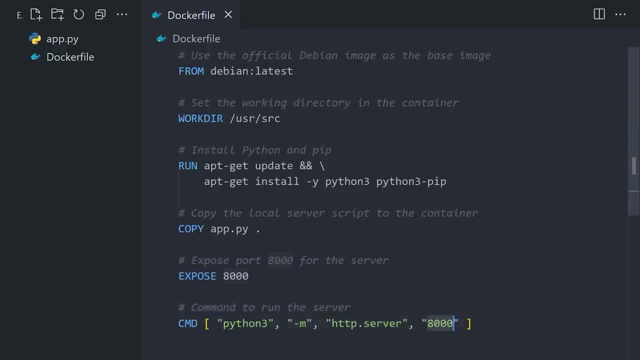 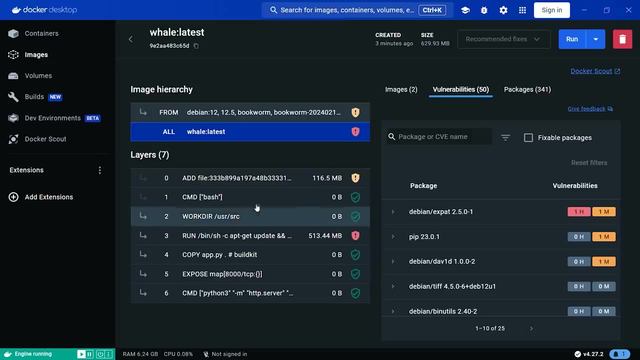 is like a blueprint that tells Docker how to configure the environment that runs your application. The Docker file is then used to build an image which contains an OS, your dependencies and your code, like a template for running your application And we can upload. 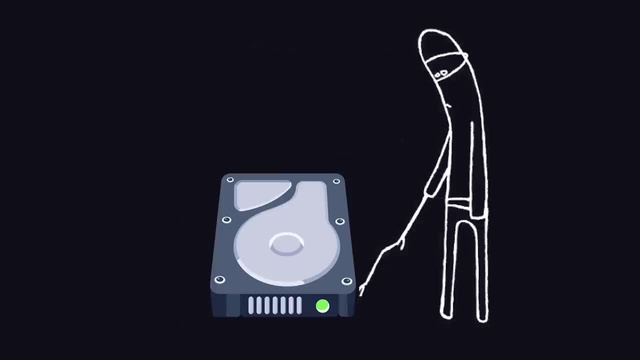 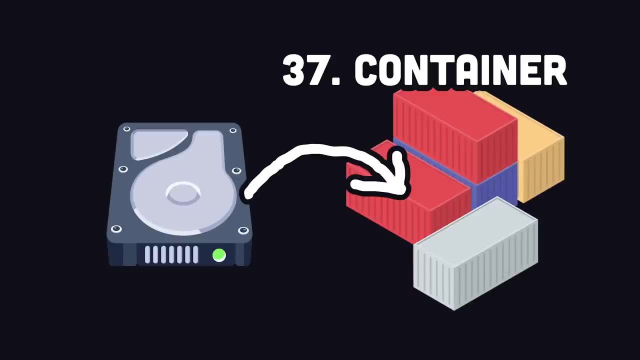 this image to the cloud, to places like Docker Hub, and share it with the world. But an image by itself doesn't do anything. You need to run it as a container, which itself is an isolated package running your code that in theory, could scale infinitely in the cloud. Containers are stateless. 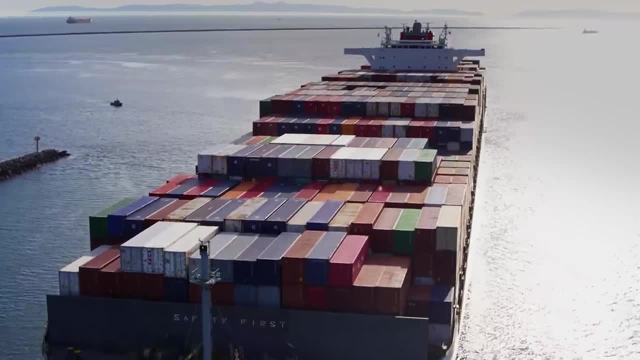 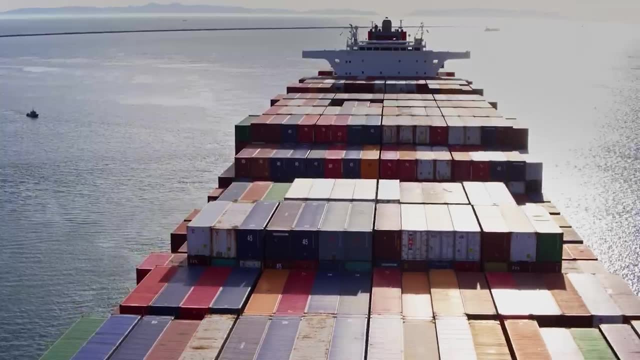 which means when they shut down, all the data inside them is lost. But that makes them portable and they can run on every major cloud platform without vendor lock-in. Pretty cool, but the best way to learn Docker is to actually run a container. Let's do that right now by creating a Docker file. 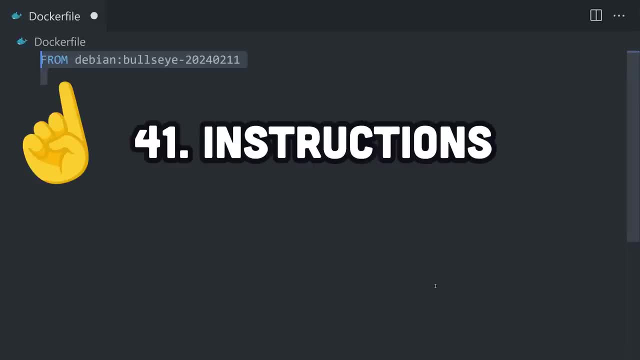 A Docker file contains a collection of instructions which, by convention, are in all caps. FROM is usually the first instruction you'll see which points to a base image to get started. This will often be a Linux distro and may be followed by a colon. 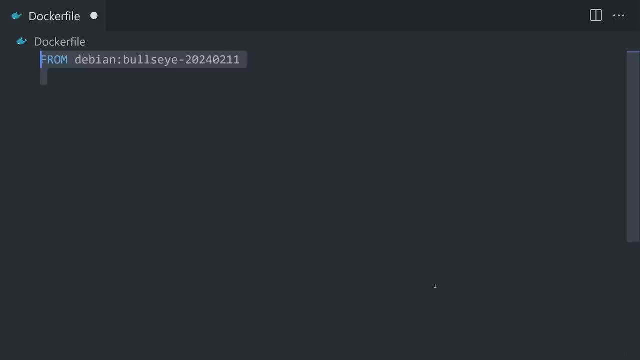 which is an optional image tag and, in this case, specifies the version of the OS. Next we have the working directory instruction, which creates a source directory and CDs into it, And that's where we'll put our source code. All commands from here on out will be executed from: 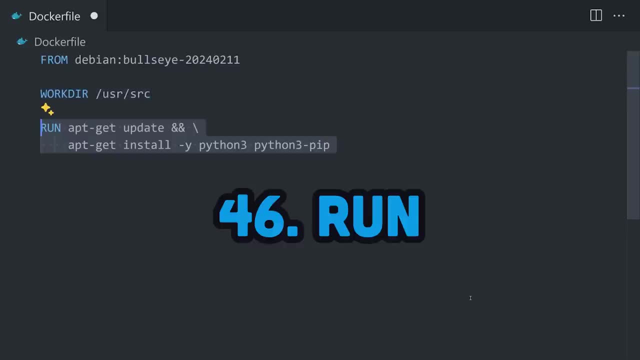 this working directory. Next, we can use the run instruction to use a Linux package manager to install our dependencies. Run lets you run any command just like you would from the command line. Currently we're running as the root user, but for better security we could also create a non-root. 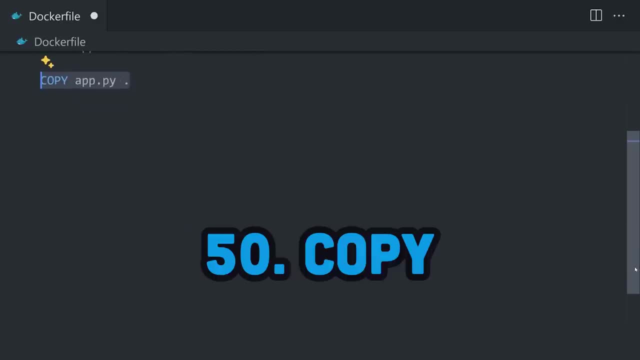 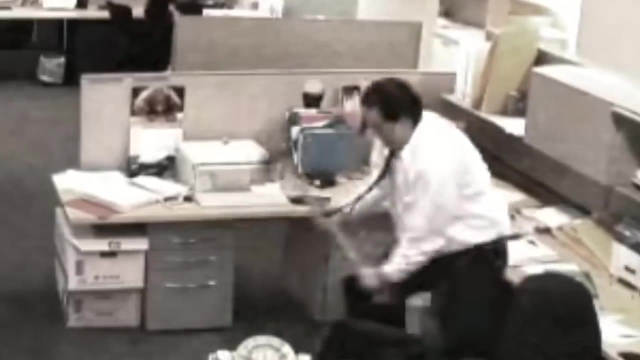 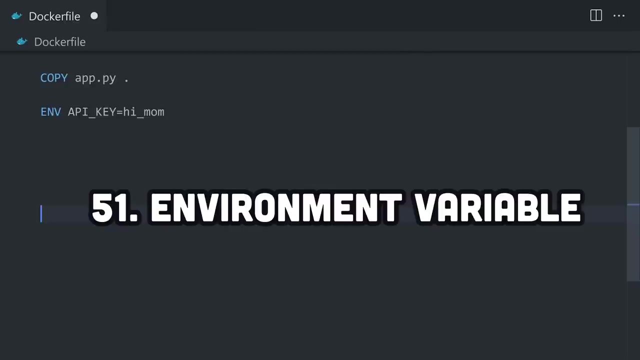 user with the user instruction. Now we can use copy to copy the code on our local machine over to the image. You're halfway there. let's take a brief intermission. Now to run this code, we have an API key which we can set as an environment variable with the. 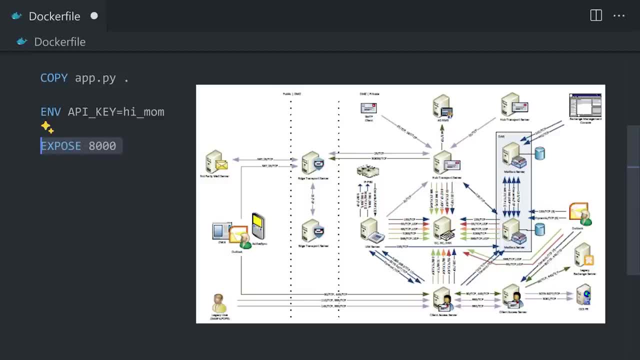 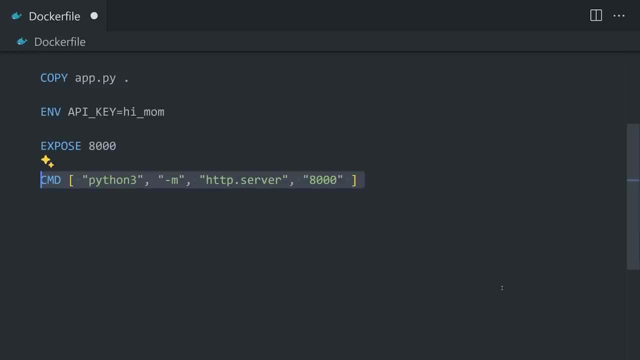 ENV instruction. We're building a web server that people can connect to, which requires a port for external traffic. Use the expose instruction to make that port accessible. Finally, that brings us to the command instruction, which is the command you want to run when starting up a. 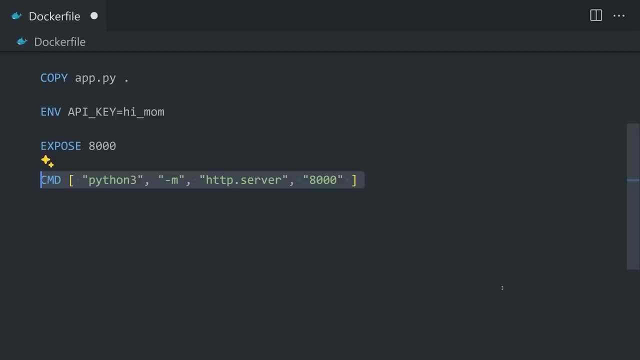 container. In this case, it will run our local machine and we'll use the command to run our web server. There can only be one command per container, although you might also add an entry point allowing you to pass arguments to the command when you run it. That's everything we. 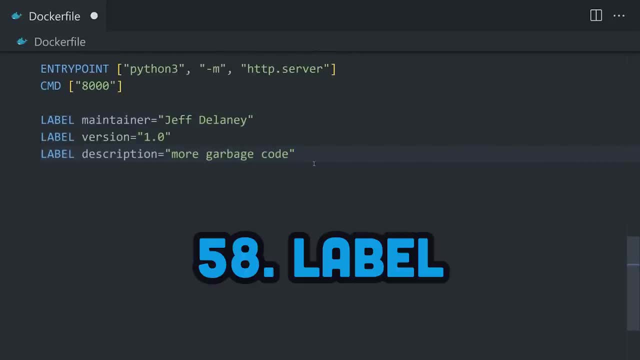 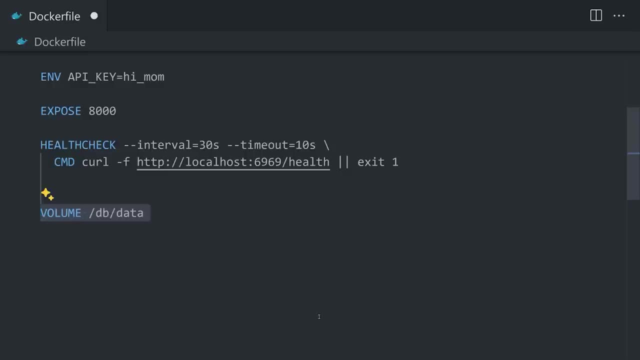 need for the Dockerfile, But as an added touch, we could also use label to add some extra metadata, or we could run a health check to make sure it's running properly. Or if the container needs to store data that's going to be used later or be used by multiple containers, we could mount a 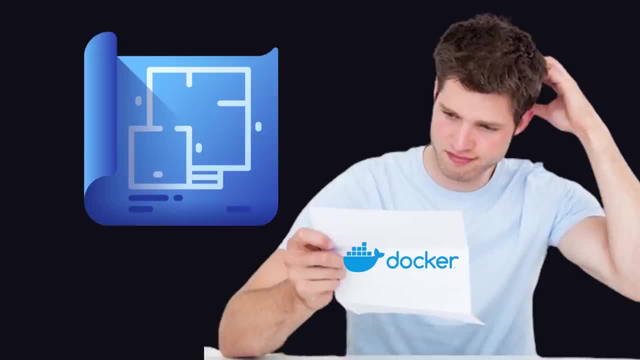 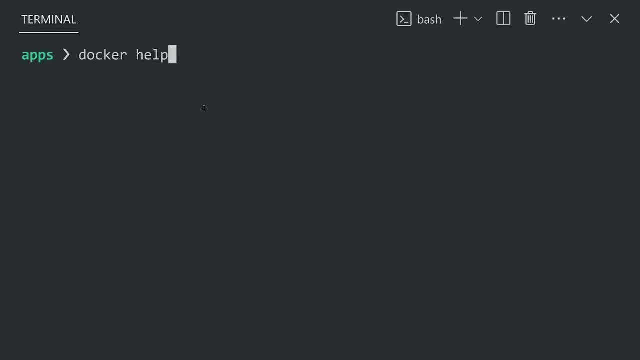 volume to it with a persistent disk. Okay, we have a Dockerfile. so now what? When you installed Docker Desktop, that also installed the Docker CLI, which you can run on the terminal Run docker. help to see all the possible commands, but the one we need right now. 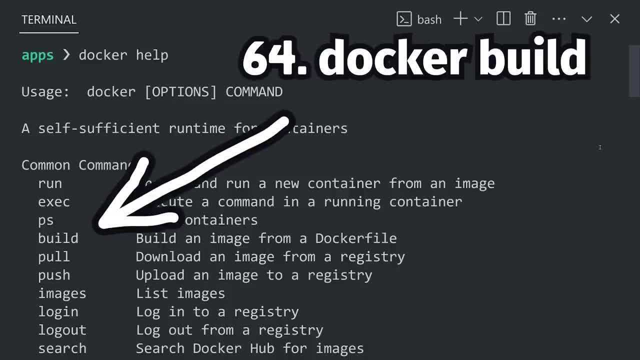 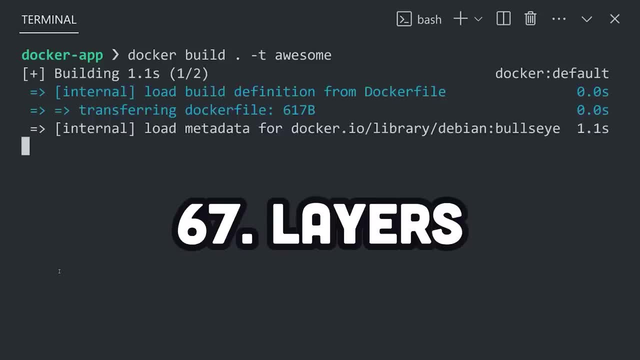 is docker build, which will turn this Dockerfile into an image. When you run the command, it's a good idea to use the T flag to tag it with a recognizable name. Notice how it builds the image in layers. Every layer is identified by a SHA-256 hash, which means if you modify your Dockerfile. 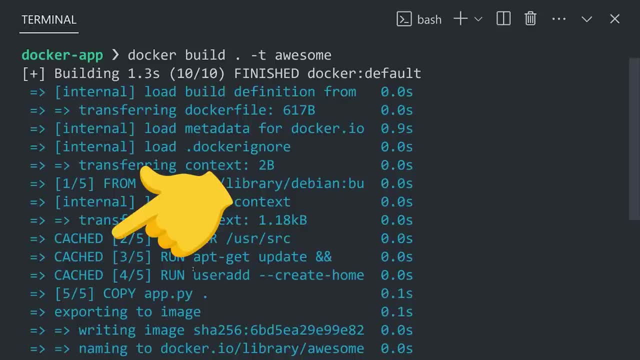 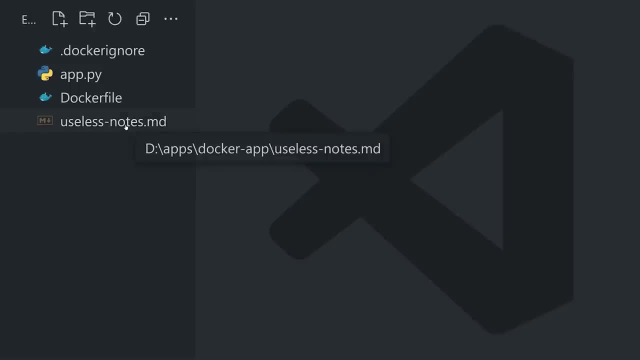 each layer will be cached, so it only has to rebuild what is actually changed, And that makes your workflow as a developer far more efficient. In addition, it's important to point out that sometimes you don't want certain files to end up in a folder, so you want to make sure that you're 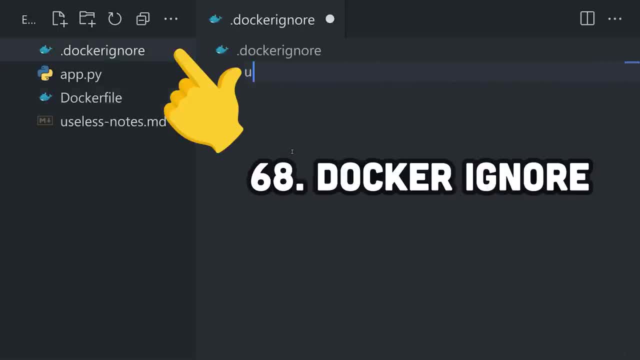 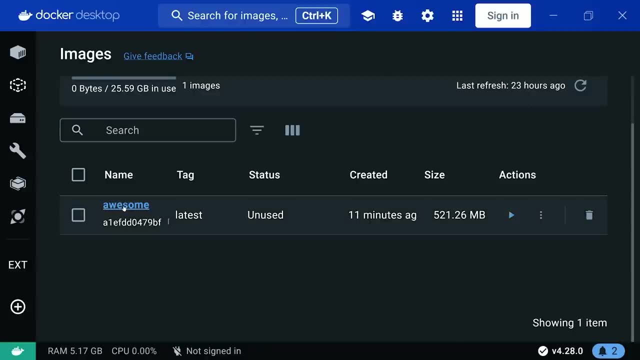 going to end up in a Docker image, in which case you can add them to the dockerignore file to exclude them from the actual files that get copied there. Now open Docker Desktop and view the image there. Not only does it give us a detailed breakdown, but, thanks to Docker Scout, we're able to proactively 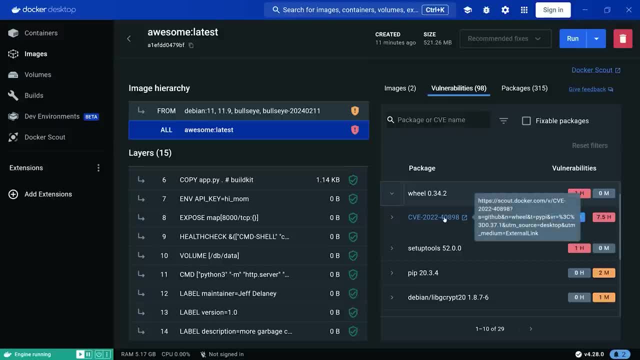 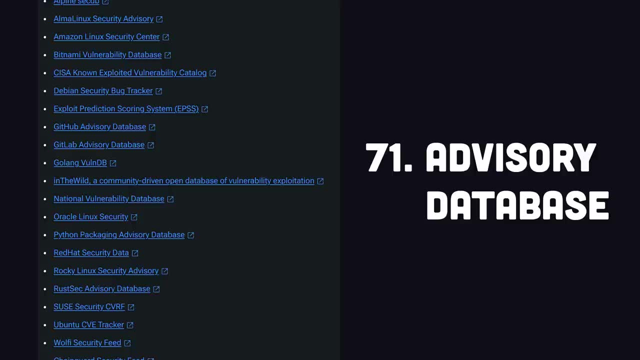 identify any security vulnerabilities for each layer of the image. It works by extracting the software bill of material from the image and compares it to a bunch of security advisory databases. When there's a match, it's given a severity rating, so you can prioritize your. 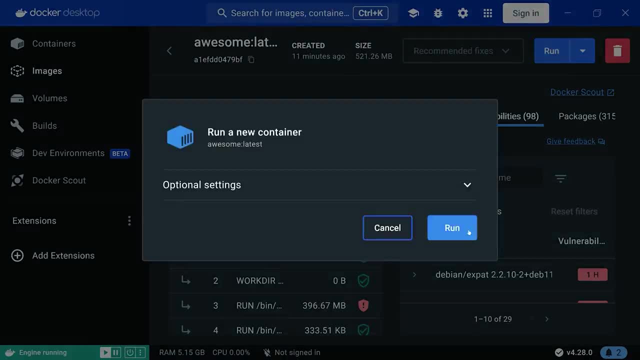 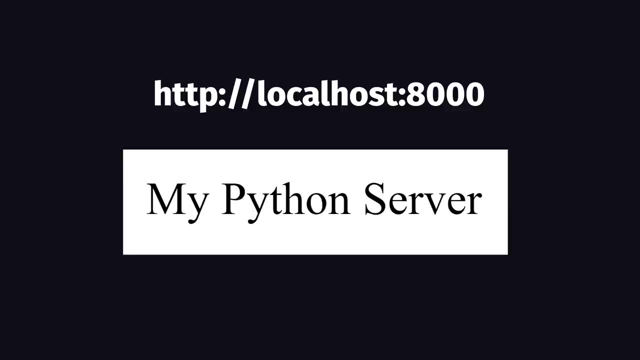 security efforts. But now the time has finally come to run a container. We can accomplish that by simply clicking on the run button Under the hood. it executes the docker run command and we can now access our server on localhost In addition. 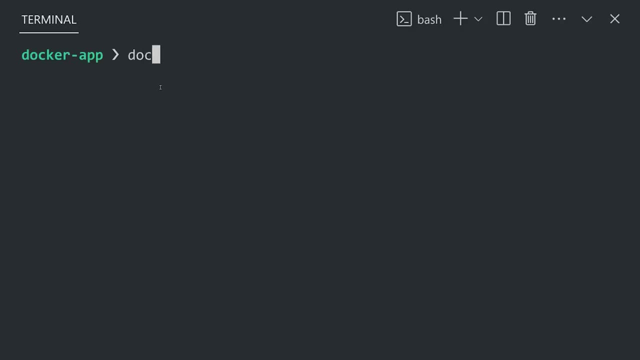 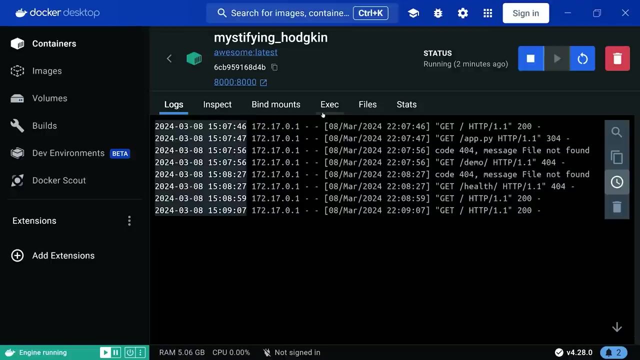 we can see the running container here in Docker Desktop, which is the equivalent to the docker ps command, which you can run from the terminal to get a breakdown of all the running and stop containers on your machine. If we click on it, though, we can inspect the logs from this container. 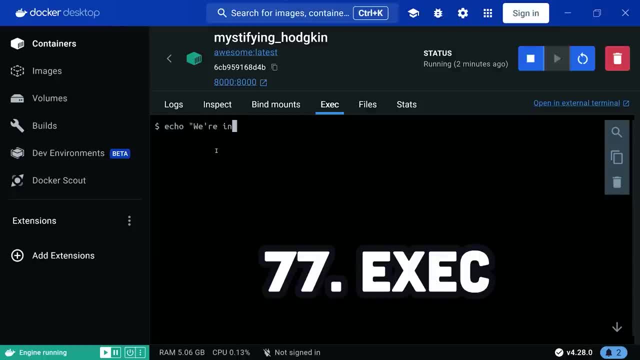 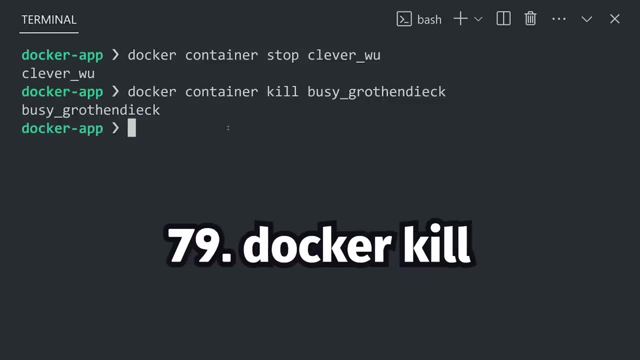 or view the file system, and we can even execute commands directly inside the running container. Now, when it comes time to shut it down, we can use docker stop to stop it gracefully, or docker kill to forcefully stop it. You can still see the shutdown container here in the UI or use remove to get rid of it. But now 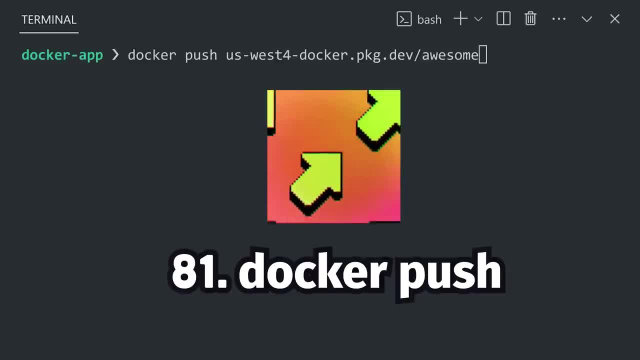 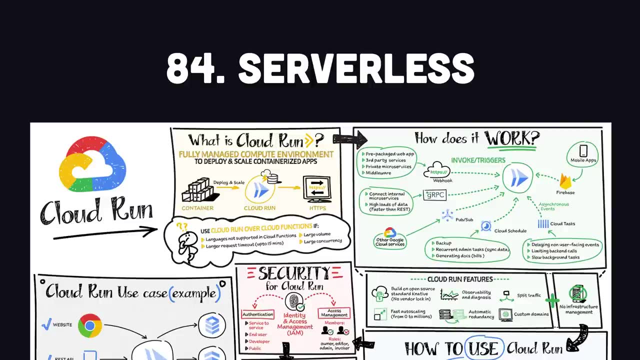 you might want to run your container in the cloud. Docker push will upload your image to a remote registry, where it can then run on a cloud like AWS with Elastic Container Service, or it can be launched on serverless platforms like Google Cloud Run. Conversely, you may want: 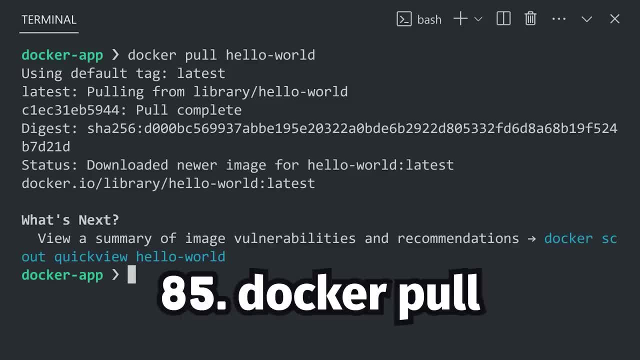 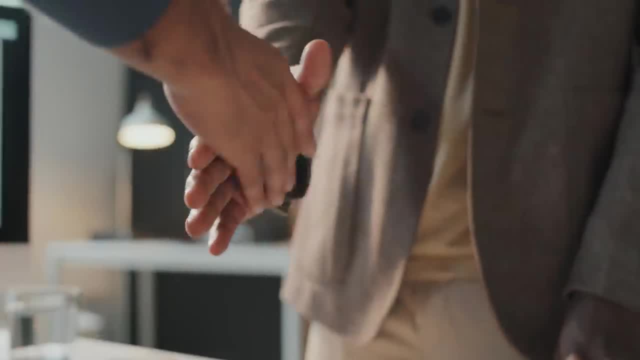 to use someone else's Docker image, which can be downloaded from the cloud with docker pull, And now you can run any developer's code without having to make any changes to your local environment or machine. Congratulations, you're now a bonafide and certified Docker expert. 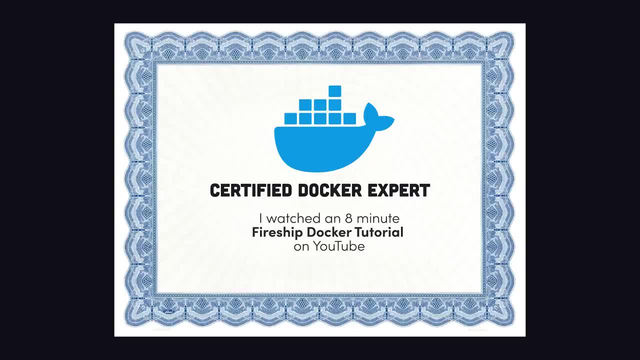 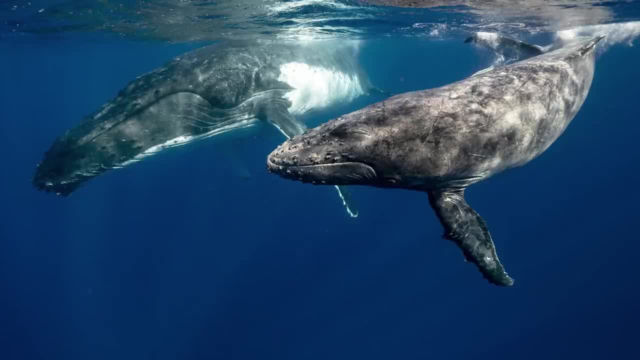 I hereby grant you permission to print out this certificate and bring it to your next job interview. But Docker itself is only the beginning. There's a good chance: your application has more than one service, in which case you'll want to know about Docker Compose, a tool for managing. 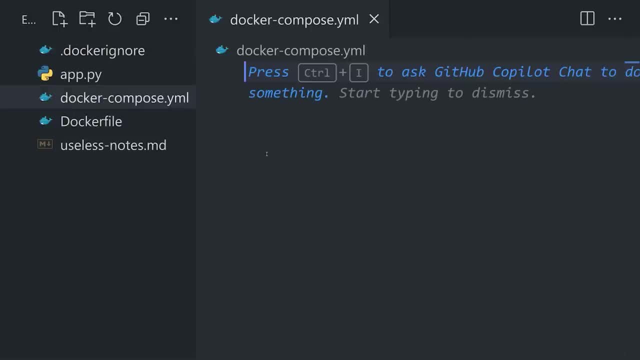 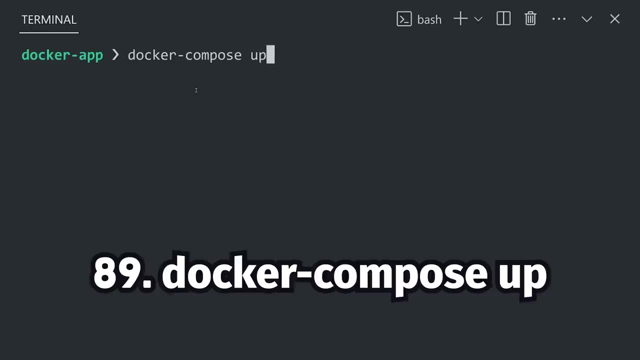 multi-container applications. It allows you to define multiple applications and their Docker images in a single YAML file, like a front-end, a back-end and a database. The Docker Compose up command will spin up all the container's data simultaneously, while the down command will stop them. That works on an individual server.